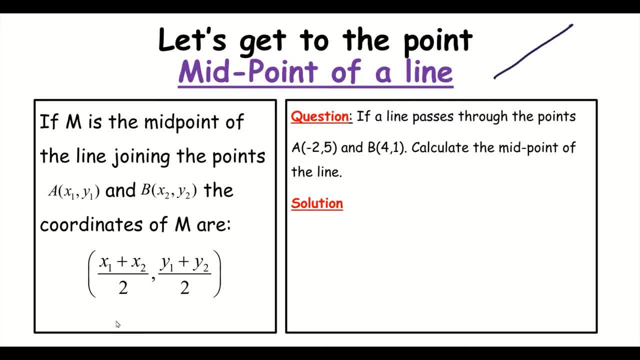 So if I have the points A and B, so A is right here and B is right here, so A is right here and B is right here- then the midpoint is going to be halfway between the points A and B. So if my A coordinates are and my B coordinates are, then the midpoint 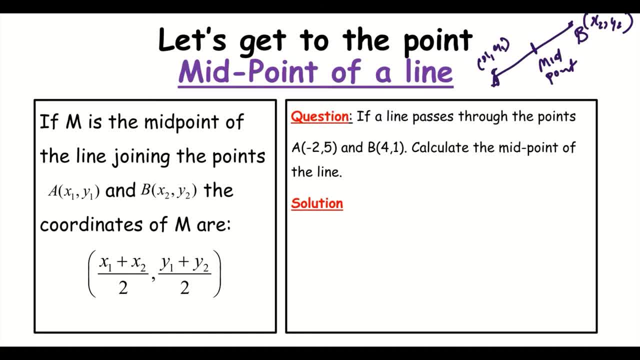 is going to be half of the sum of the X part of the coordinates and the Y part of the coordinates. So let's look at an example. Look at the points A and B. Calculate the midpoint of the line. Now, for some students, they may need to identify what their X1 and Y1 is going to be, or what their Y2. 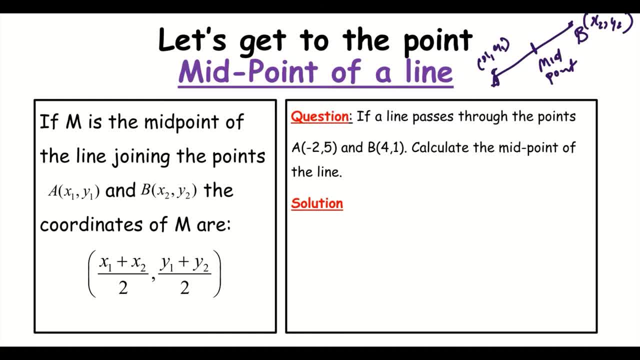 and X2 is going to be. Now, in the case of a midpoint, it's not significant because multiplication and addition are commutative. Hence, any how you set the midpoint, it's not significant. Hence, any how you set the midpoint, it's not significant, because multiplication and 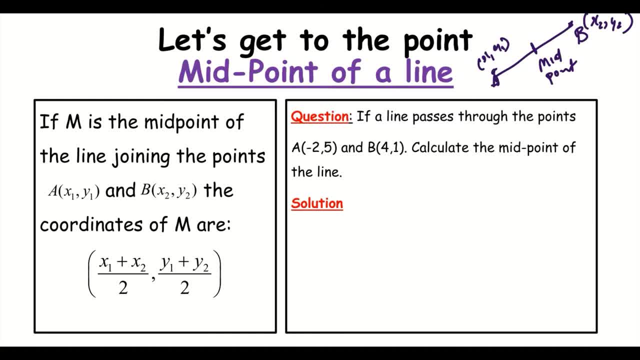 addition are commutative. Hence, any how you set the midpoint, it's not significant, because multiplication and addition are commutative. Now, some students may want to set it in this fashion, but I don't have any idea what your big 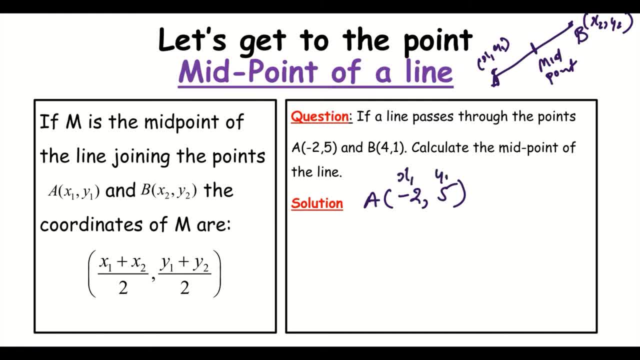 is going to be SO in this case. that would be a bunch of sheets of paper, So you will want to set the X part And the Y part. you will get about the same value, But for some students and for the sake of this video, I will highlight the X1, and the. 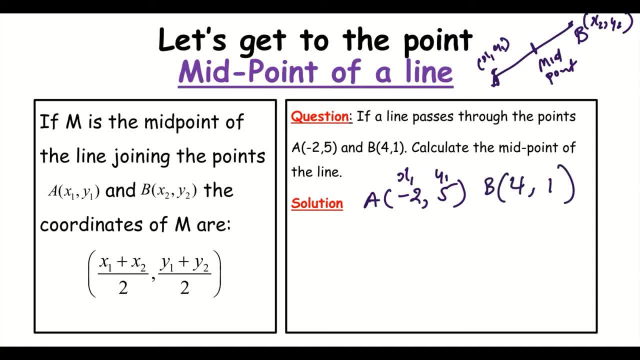 Y1 and the X2, and the Y2.. So we have the points A, so this cancels the Y1 and the Y2.. Then we have B is, So we can select four obsessions and they're what they are, And now we are going to have stakeholders for 37 of them. So in this case, if I spell, 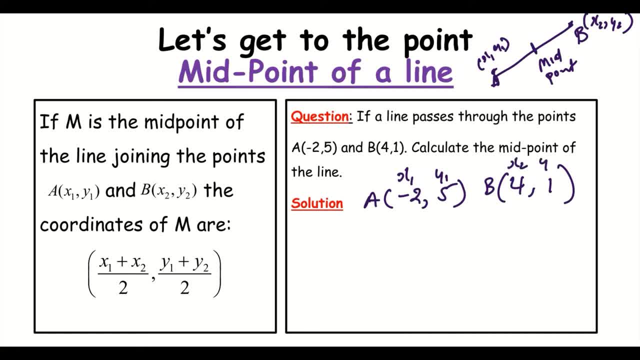 4 b over x2 y2 and you could interchange them still wouldn't make a difference. you could make this a be the x2- y2 and let b be the b1, sorry, be the x1 y1. it's still not going to change the answer. so hence the midpoint is equal to add our both x's negative 2 plus. 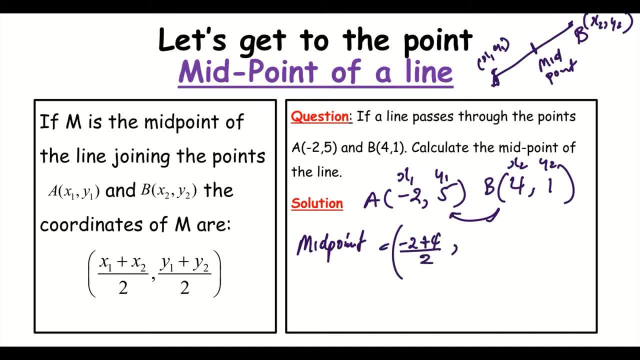 4 divided by 2 comma, 5 plus 1 divided by 2, now midpoint is equal to negative. 2 plus 4 gives us positive. 2 divided by 2 and plus 5 gives us 6 over 2. so the midpoint is equal to 1- 3. so the coordinates for the midpoint are 1- 3. so if I were to draw the 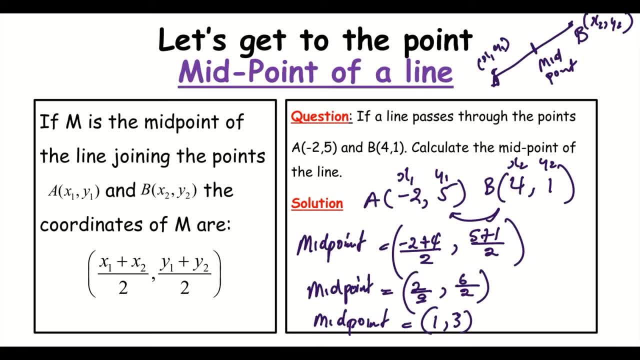 points negative: 2, 5 and 4: 1 on a graph. if I'm to bisect that line in two, if I'm to find that line halfway, it's going to be at the point 1- 3. so for the midpoint formula we use x1 plus x2 or x2 plus x1 divided. 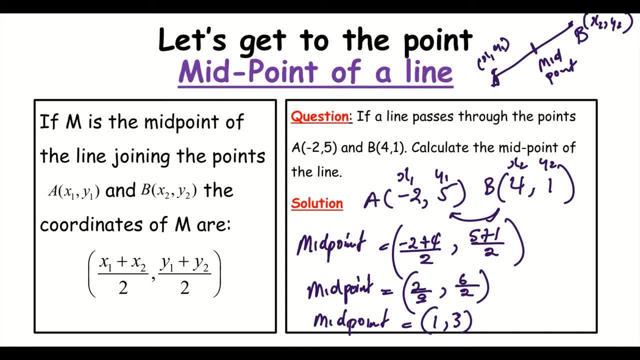 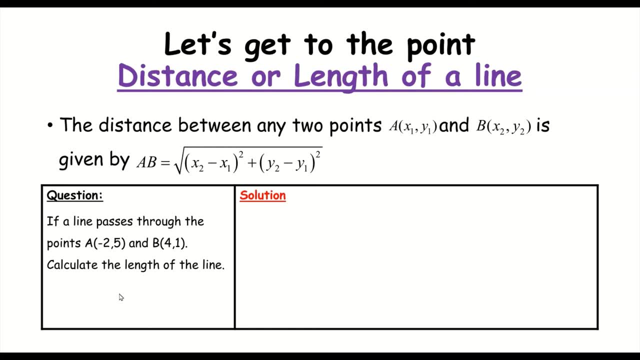 by 2 comma: y1 plus y2 or y2 plus y1 divided by 2. now if we want to find the length of a straight line passing through any two points on the same line, then we can use the formula square root: x2 minus x1, r squared plus y2 minus y1. 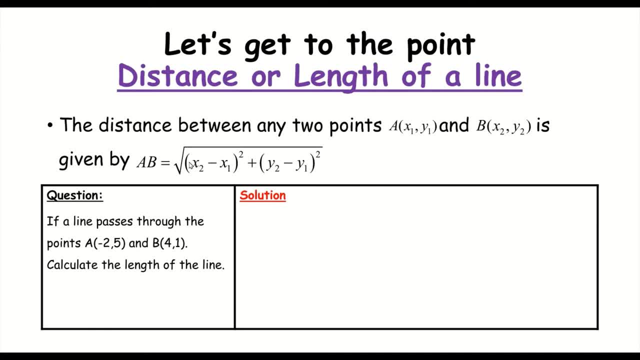 r squared now. the order doesn't matter. if you put x1 before x2 or x2 before x1, it's still not going to change x1 bad. So it's still positive. 2 minus x2 minus y1, all squared now. the order doesn't matter. if you put x1 before x2 or x2 before x1, it's still not going to change the answer. now see the dengan vernacular value is the same with the leaders. if you bend the other way, a little to the right and in order to get that, if you bend the other way also, there'll be a där in between six, so 8. over this and over here you can see the difference. 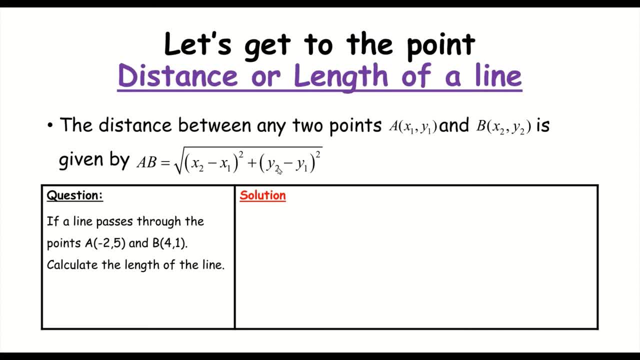 it's still not going to change the answer because everything is going to come out all squared. and if you have y1 before y2, it still won't change your result because everything will come out all squared. now question: if a line passes through the points a, negative 2, 5 and b 4, 1 calculate. 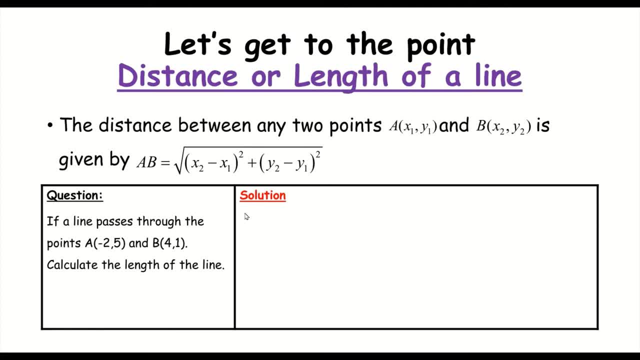 the length of the line. now we still need to establish. for some persons we can establish what is our x 1 and our x 2 or y 2, 1 or y 1. so, given the coordinates, a is equal to negative 2, 5. 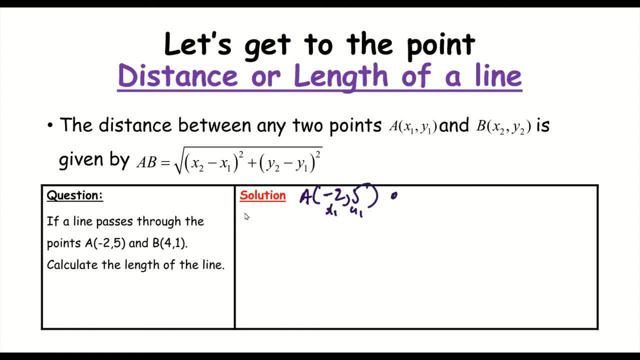 that's my x 1, y 1, and b is 4, 1 and this would be my x 2, y 2. so we're now going to substitute the values into our formula. so we're going to substitute values. so we now have a. b is equal to the square root of x- 2, which is our 4. 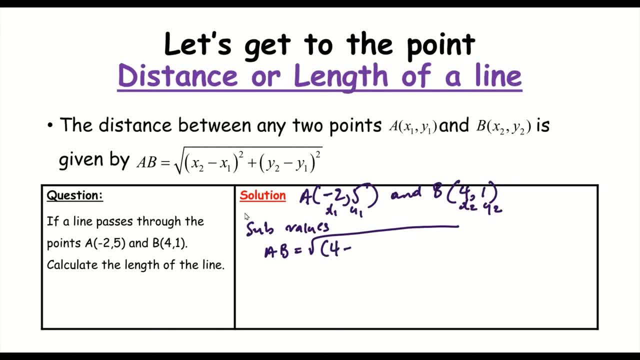 minus x, 1, which is negative, 2 all squared, plus y 2, which is equal to 1, minus y 1, which is 5 all squared. so we have a. b is equal to the square root of 4 minus negative 2, gives us: 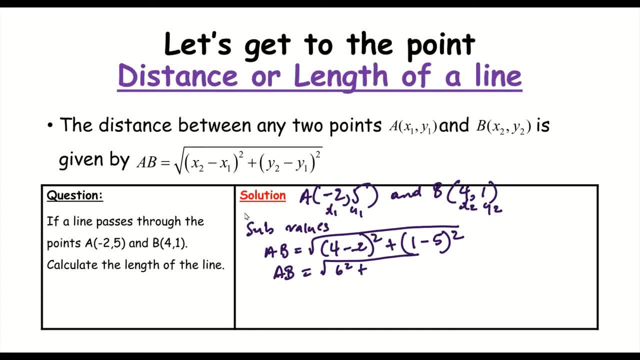 6, so we get 6 square. plus 1. minus 5 gives us negative 4 all square. so a b is equal to the square root of 6 squares. with the same thing i've seen six times six: the gives us 36 and negative 4 times negative 4 gives us 16.. so now we can go ahead and add 36 plus 16. 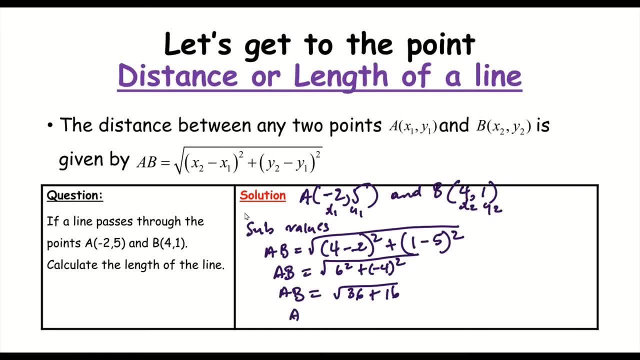 and that gives us square root 52. so a- b is equal to the square root of 52 and because it's a length or because it's distance, say 52 units. now let us look at if we had let um x1 go before x2 and y1 go before y2, what would have happened? so we could say a- b. 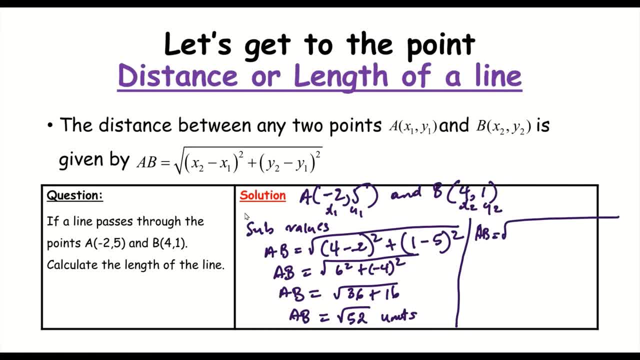 is equal to the same square root and our. this time we're going to say y1 minus y2 and x1 minus x2. so the square root of x1 would be negative: 2 minus 4 plus y2- sorry y1, which would be 5 minus 1 all squared. so we have a. b is equal to the square root of. 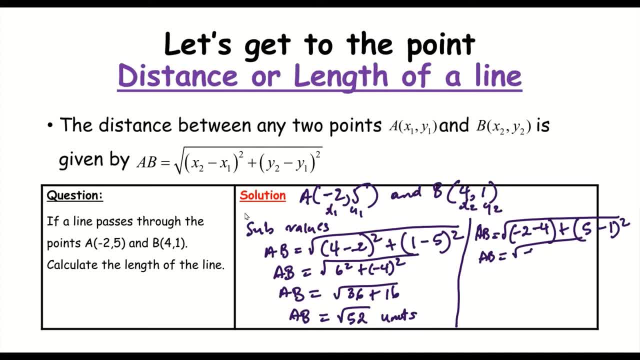 negative. 2 minus 4 gives us negative 6 all squared. plus 5 minus 1 is 4 all squared. so we still get a. b is equal to the square root of 36 plus 16.. so AB is equal to square root 52.. 52 units would be our final answer. 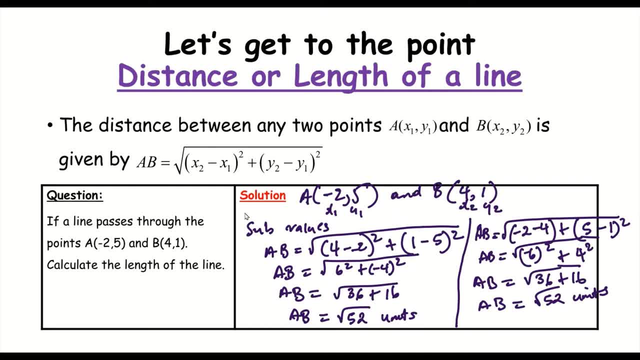 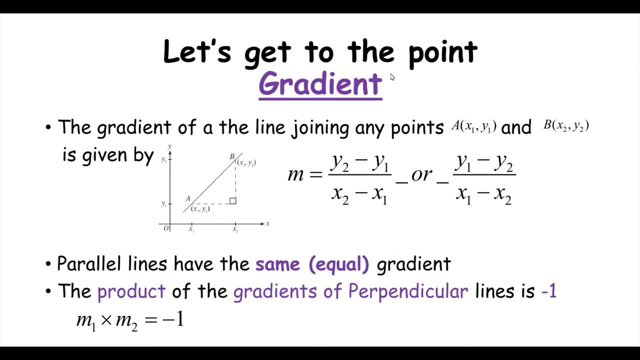 Or if you want to write your answer as a decimal, you can go ahead and do so. Now, the gradient of a line is the rate at which it goes upwards or downwards. Another name for gradient is slope. Now the slope can either be positive or negative. 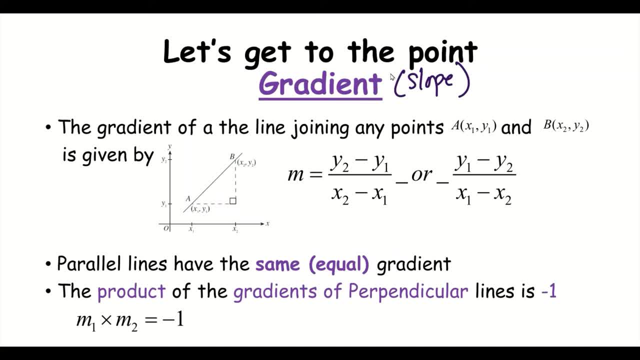 And the sign indicates whether the line slopes upwards or downwards from left to right. So this would be a negative gradient, This would be a positive gradient, And a horizontal line would mean that our gradient is equal to zero. Now the symbol that we use for gradient is: 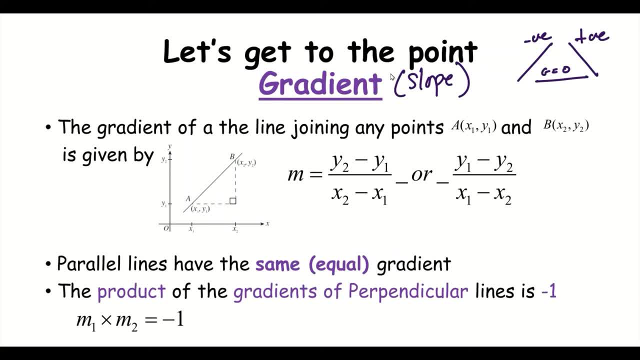 Small m, Small m, and we use capital M for midpoint and common m for gradient. The formula that we're going to use is y2 minus y1 over x2 minus x1. Or, as I said earlier, it doesn't matter if you want to put the y1 before the y2 or the x1 before the x2.. 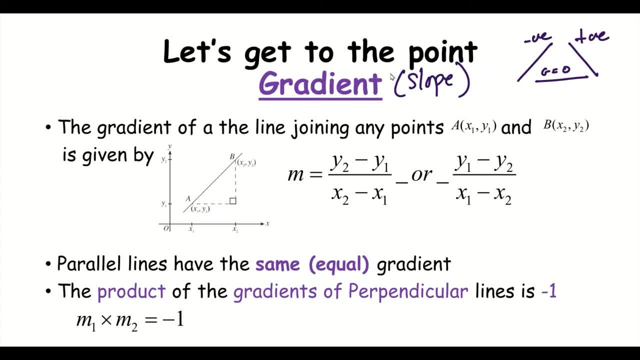 The sign is what is important. The sign will come out the same in the end. So key pointers to note: Parallel lines have the same or equal gradient And the product of the gradient of perpendicular lines is 1.. I'll use the formula. 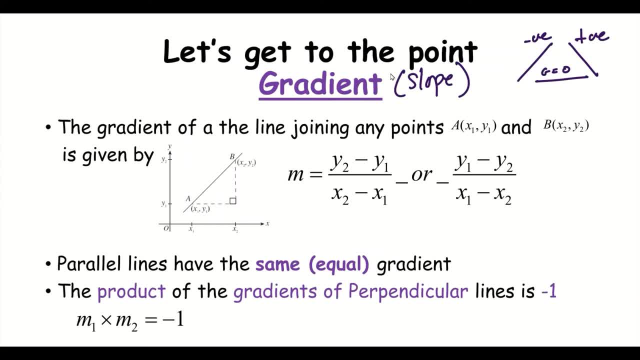 m1 times m2 is equal to negative 1.. So if I know the gradient of a perpendicular line to my line, to the original line, when I multiply both gradients, I'm going to get, I'm going to get my negative 1.. 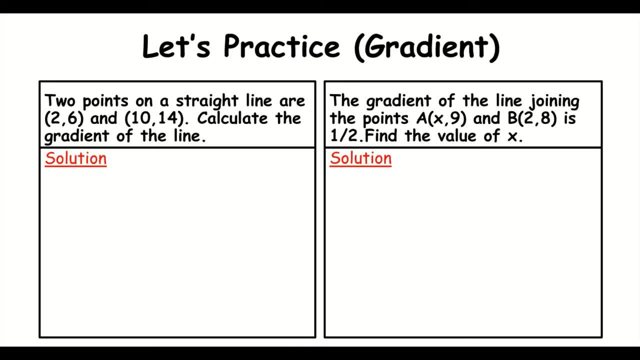 Now let's practice the concept of gradient with these two questions. So two points on a straight line are 2, 6 and 10, 14.. Calculate the gradient of the line. So we know that the gradient formula is: 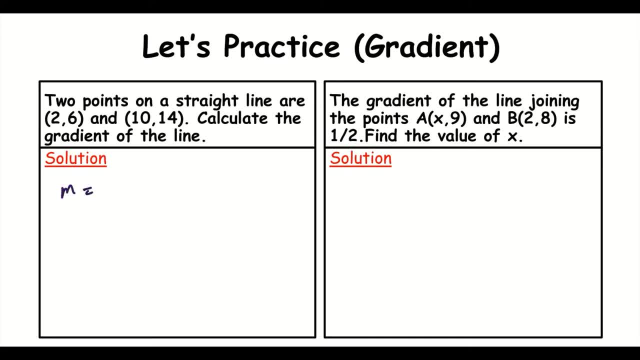 m. common m is equal to y2 minus y1 over x2 minus x1. x1. Or we could stick to y1 minus y2 or x1 minus x2.. It doesn't matter which one of the formulas you want to use. 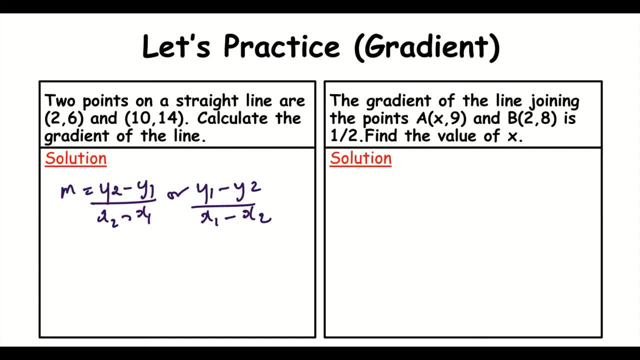 Still going to be the same answer. Hence m is equal to. Let's establish what our x1, y1, x2, y2.. So we have y2.. So which is 14 minus y1 is 6 over. x2 is 10 minus y1 is 2.. 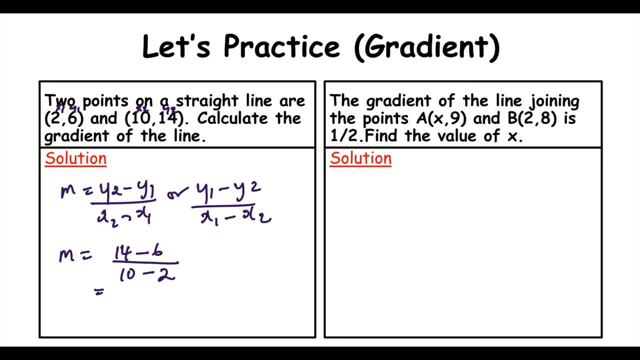 So we have: 14 minus 6 gives us 8, and 10 minus 2 gives us 8.. So our gradient is equal to 8 divided by 8, 1.. So we have. So we have. 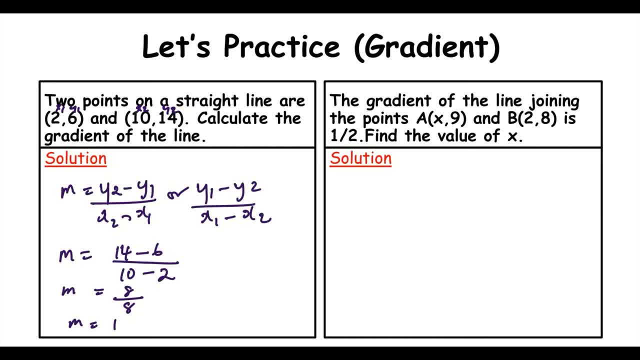 Then in our next question, the gradient of a line joining the points a, x9.. So we have an unknown here. And b, 2, 8 is a half Calculate the value of x. So it's an application question where we already know the gradient. 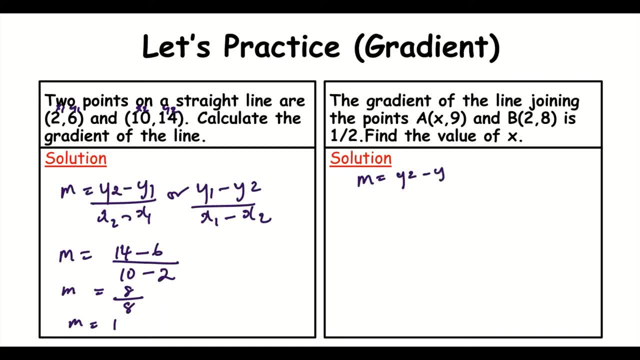 So m is equal to y2 minus y1 over x2 minus x1.. Now we have- Now we already know- the value of our m, but one of our values for x over x1 is going to be missing. So let's plug in what we have first. 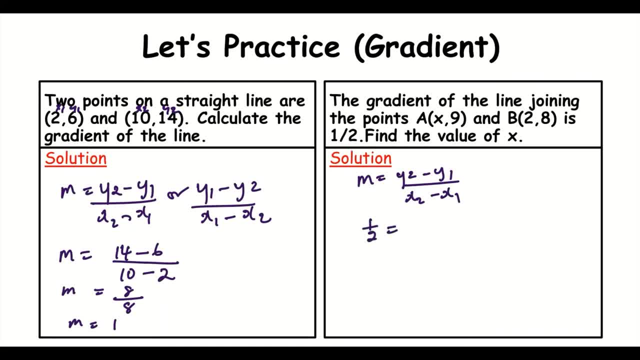 So m is equal to a half. Let's identify this would be over x1, y1, x2, y2.. So we have y2, which is 8 minus 9, over x2.. x2,, which is 2 minus 9, or x1 is x. 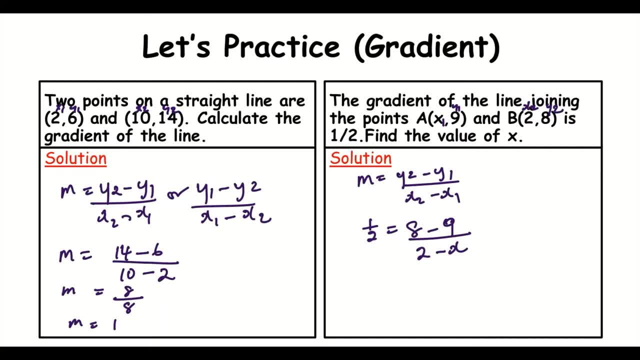 So we can keep it as that. Now we can do what we call cross multiplication in some cases where we can easily- Let me just write it a little better- We can cross multiply to find the value. So let's simplify this some more. 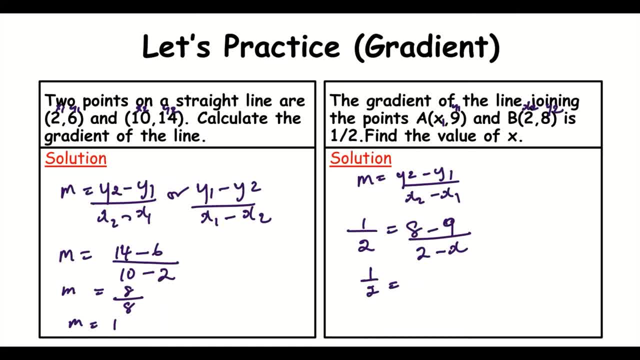 So half is equal to 8 minus 9 gives us negative 1.. So let's simplify this some more, So we can apply our cross multiplication concept, And then we have 2 minus x times 1 will give you back 2 minus x. 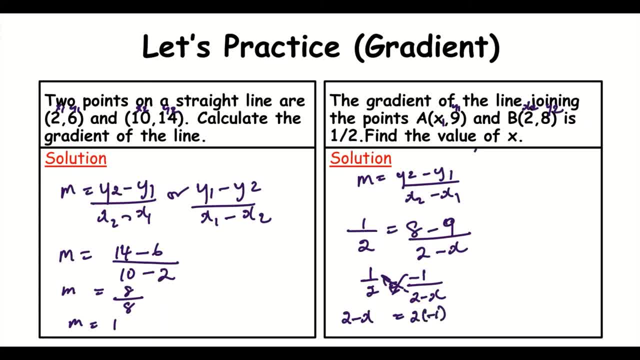 And then we're going to have 2 times negative 1. So we now have: 2 minus x is equal to negative 2. We're going to apply solving for equations, solving for x. So we have negative. x is equal to negative 2 minus 2.. 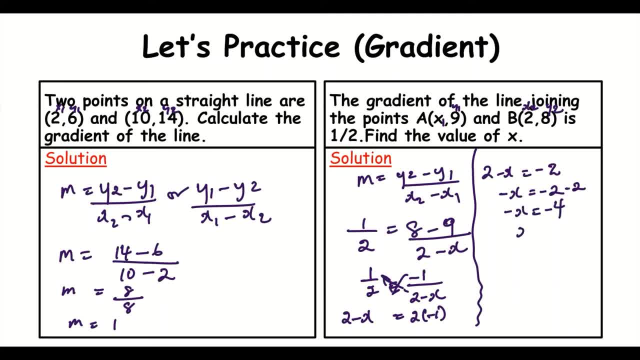 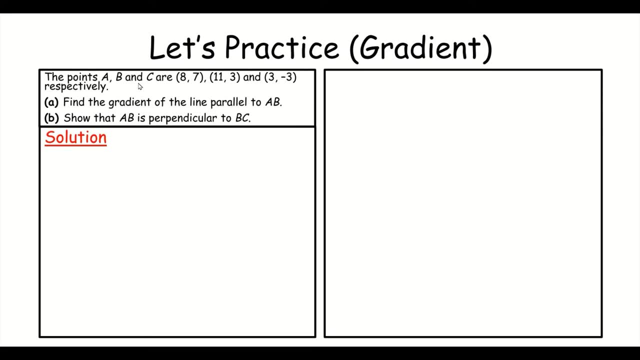 So negative x is equal to negative, 4. x is equal to positive 4. So therefore, the value of our x is equal to 4.. Now another question. The points a, b and c are 8,, 7,, 11,, 3, and 3, negative 3.. 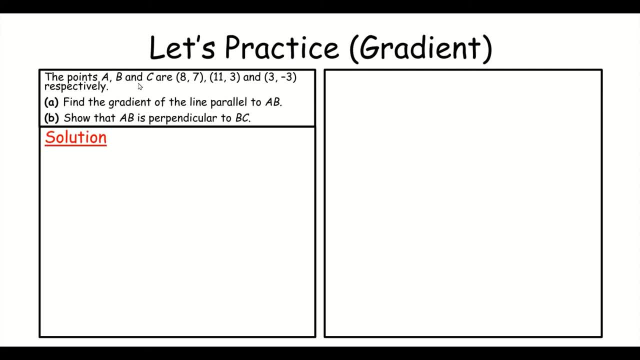 Respectively. And we know that respectively means the first point would be 8,, 7.. The second point, which is b, which is 11, 3.. And the third point, which would be 3, negative 3.. 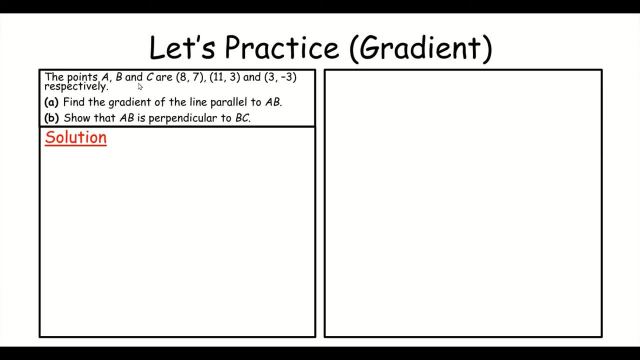 Now find the gradient of the line parallel to a- b. Now what do we know about the keyword parallel? here, Parallel lines have the same gradient. Hence, finding the gradient of a- b is finding the gradient of any other line that is parallel to a- b. 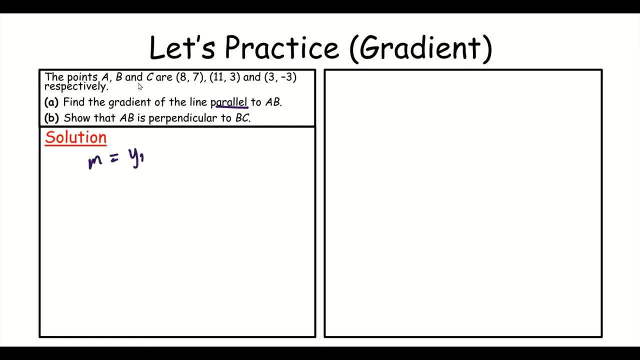 Hence gradient is equal to y1 minus y2 over x1 minus x2.. I'm using the 1, subtract the 2's in this case. here It doesn't make a difference. So m would be equal to what's our points. 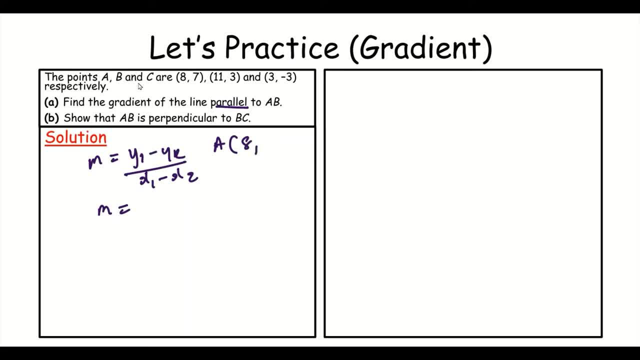 Using the points a and a is 8, 7, and b is 11, 3.. So this would be my x1, y1, x2.. So hence I can say 7 minus 3.. 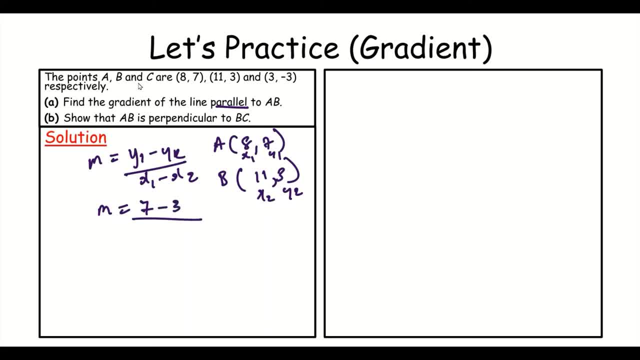 So 7 minus 3 over 8 minus 11.. So m is equal to 7 minus 3, 4. And 8 minus 11, negative 3. So our gradient would be negative 4 over 3.. 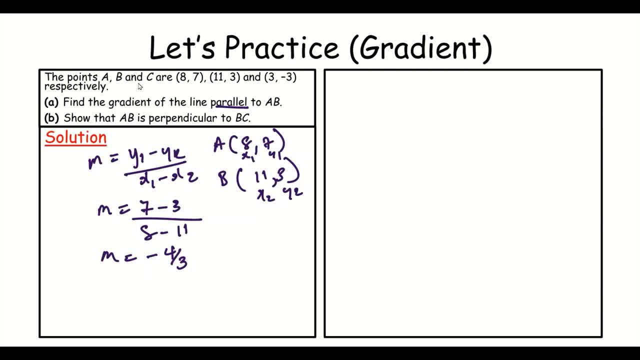 Hence, therefore, the gradient of any other line, Now the line parallel to a b, is going to be negative, 4 over 3.. So the gradient of any line parallel to a b is negative, 4 over 3.. 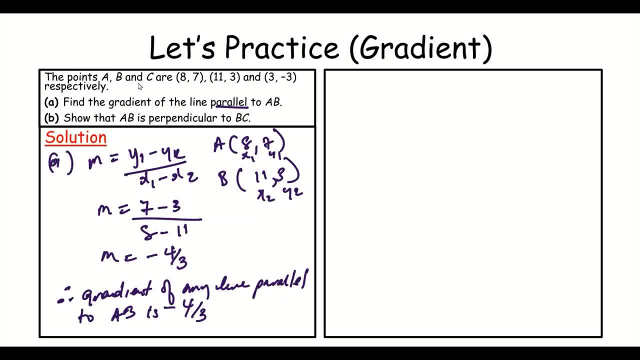 Now part b asks us to show that a- b is perpendicular. Now part b asks us to show that a- b is perpendicular to b c. Now this could be proved using other concepts like Pythagoras' theory and stuff. 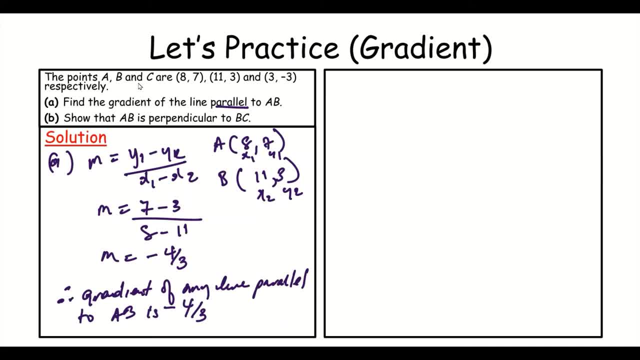 But for the sake of gradient, we'll stick to gradient. Now, what do we know about perpendicular lines? Now, perpendicular lines, their gradient, when multiplied, comes to negative 1.. So if we know the gradient of a, b, 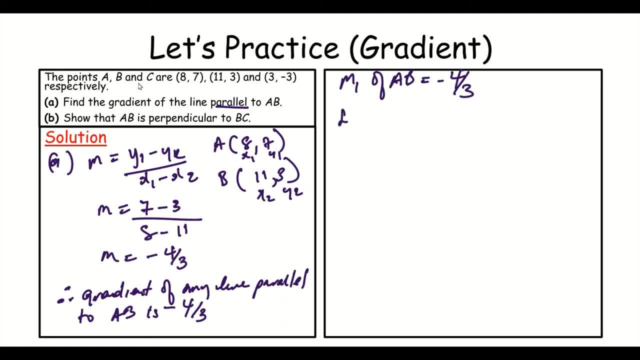 that's negative 4 over 3.. Now let's find the gradient of b c. That would be great. Let's call it m2. And let's calculate that. So that's going to be our y1 minus y2 over x1 minus x2.. 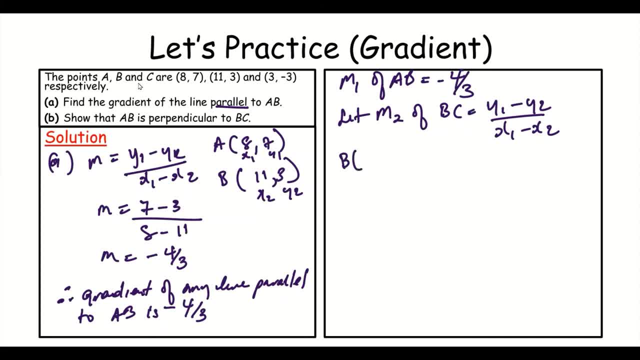 Now let's write out the points b and c. So b would be 11, 3.. And c is 3, negative 3.. That could be my x1, y1, x2, y2.. So hence gradient. 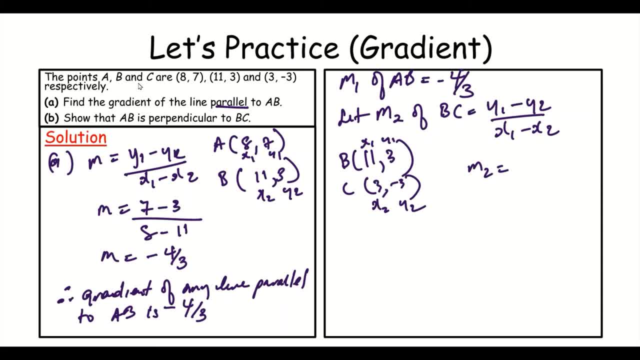 So we can have 3 minus negative 3 over. we now have 11 minus 3.. So that's going to give me 3 minus negative 3.. That's going to give me 6 over 11 minus 3.. 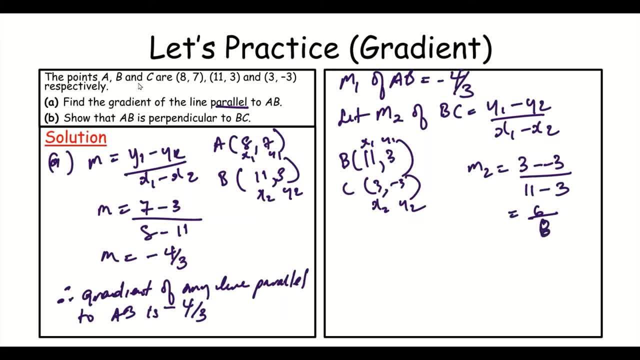 That gives me 8. Hence we can reduce our fraction to give us 3 over 4.. Now the thing is for them to be perpendicular. the product m1 times m2 must be negative 1. So let's multiply them and see what we get. 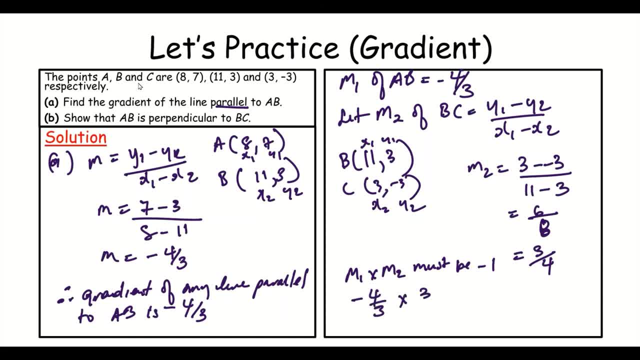 Negative: 4 over 3.. Times 3 over 4 equals. let's break it down: 4 into itself, 1, 4 into negative. 4 goes negative, 1, 3 into itself, 1, 3 into itself, 1.. 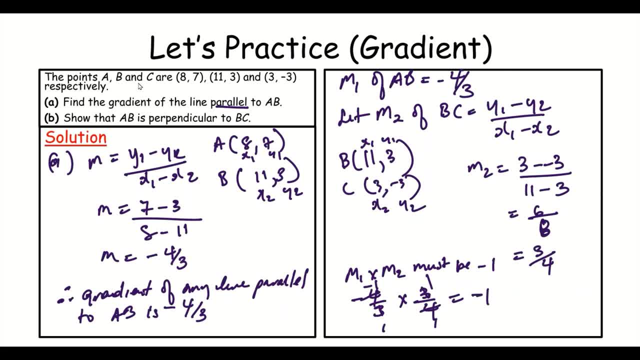 So our final answer is negative 1.. So once the product gives us negative 1, we can say: therefore they are perpendicular. So the products of a, a b times b, c is negative 1. And it's the product of the gradient, not just product, the product of the gradient. 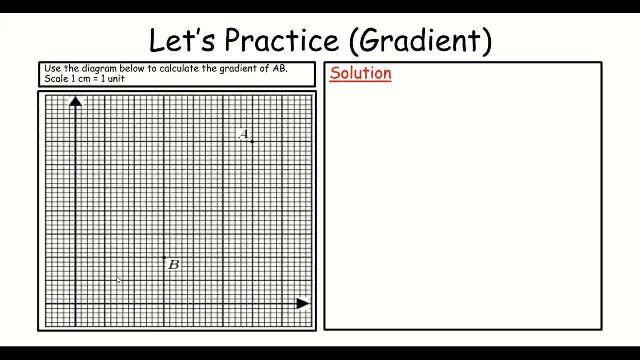 Now our final question. in this video, Use the diagram below to calculate the gradient of a, b and the scale is 1 centimeter gives us 1 unit, So calculate Now. we could calculate the gradient using rise over run, or we could identify the coordinates b and a and use our formula. 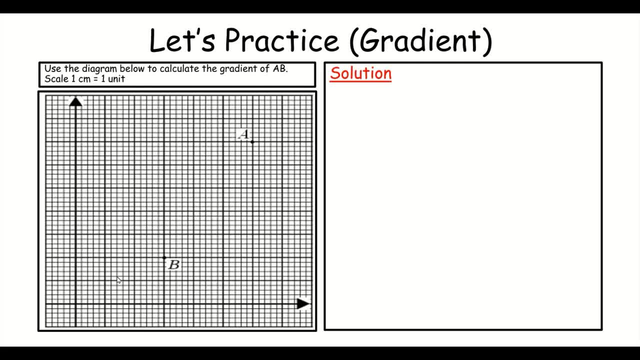 Any way you want to use it, no problem. But for the case of using rise over run, because gradient is also equal to the rise over the run. So when you have the diagrams it's just quicker to use the rise over run concept. 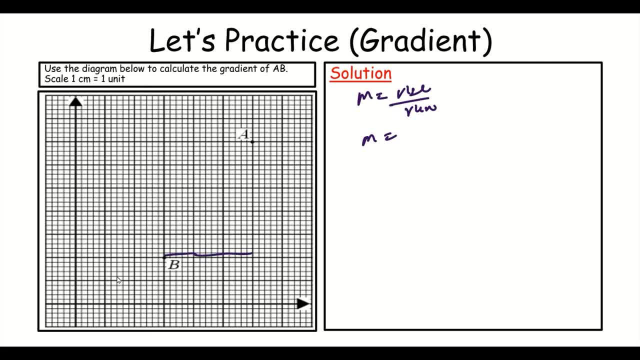 So if I'm here, 1 place, 2,, 3 places on my run. So I'm going, my run is going to be 3 and my rise is going to be 1,, 2,, 3,, 4,, 5.. 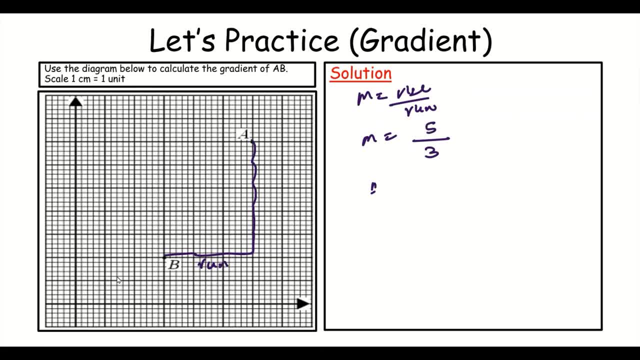 5 places up. So my gradient is going to be m is going to be equal to 5 over 3.. So you'll find it's a triangle normally And you're getting that. it's a rise over your run. 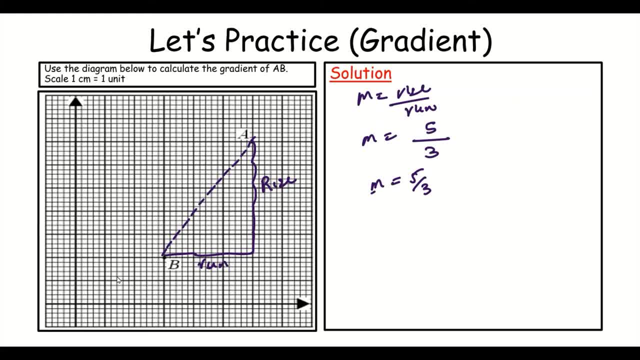 Or we could identify the coordinates of b. What would be the coordinates of b If 1 centimeter is 1, and here would be 1, then here would be 2,, then here would be 3,, here would be 1,, 2,, 3,, 4,, 5,, 6,, 7.. 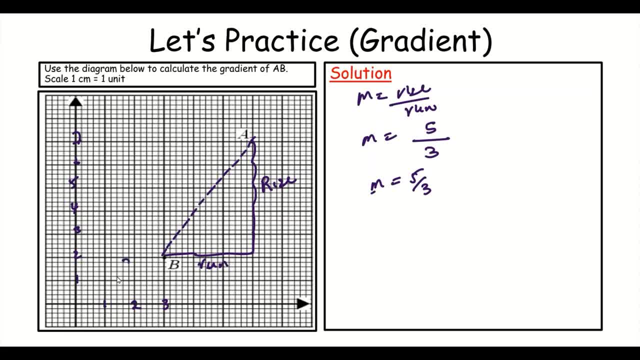 So we'll have: b would be 3, 2 and a would be 3, 4,, 5, 6, a would be 6, 7.. So we could use. We could use it also with our y2 minus y1 concept. 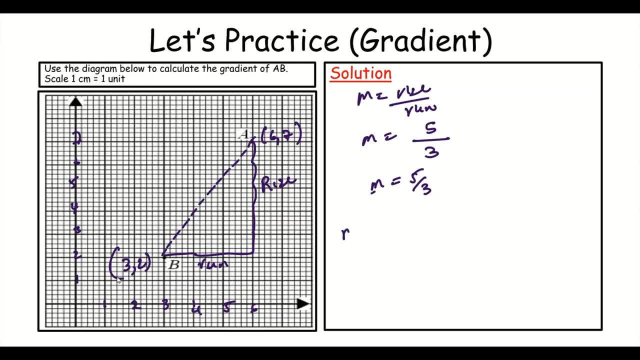 So we could test it and say: m let this be our x1, y1,, let this be our x2, y2.. We should get the same answer. We will get the same answer. Hence, let's go again. 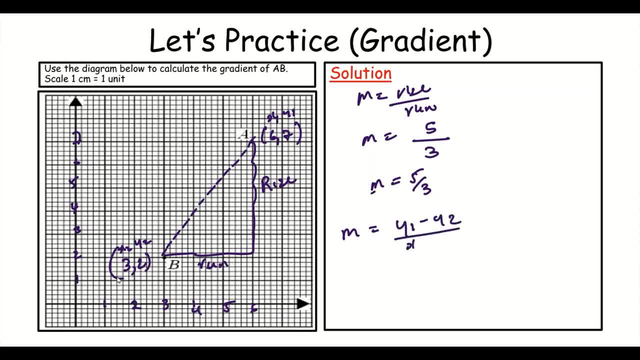 So say y1 minus y2 over x1 minus x2.. Sorry about that, It's x1 minus x2.. Hence m. What's my y1?? That's going to be 7 minus 2 over. What's my x1?? 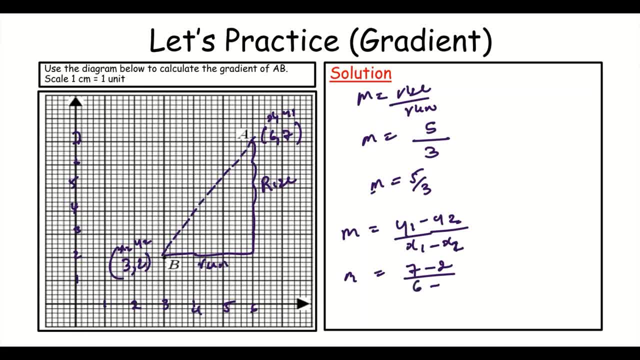 My x1 is going to be 6 minus 3.. So we have We have 5 over 3.. It doesn't matter which way you choose to do it: Gradients would be the gradients. Thank you guys for watching.